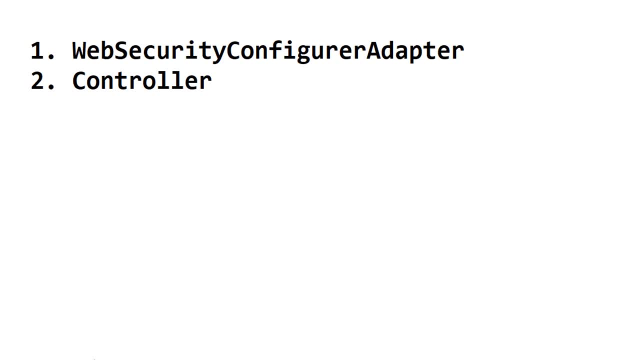 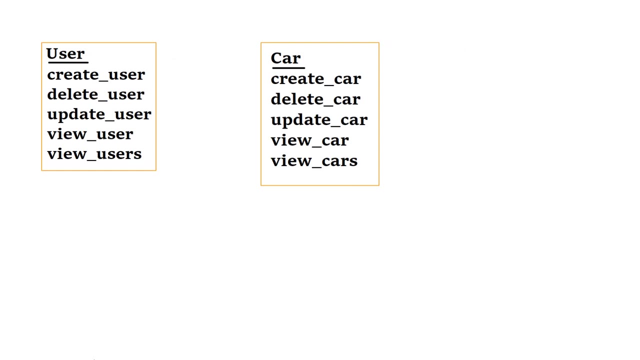 in web security configurator adapter or by using the global method security in controllers. We can see both the methods here. First, we have to understand what is role based access control. In our application we are going to use two domain objects: user and car. Car is an actual resource which we are going to access through our REST API. Five operations can be done on this car object. That is, you can create a car object. 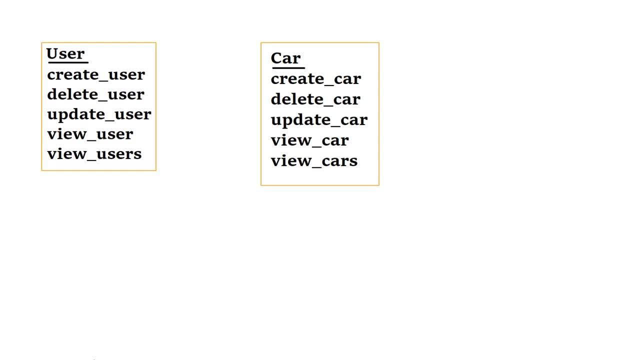 You can create your own car object. You can create and accessas for our REST API as well. You can set a result New, delete that. set the result New and view the result starting withing the ID bar. You can create a unique car with different states And you can even 국 and 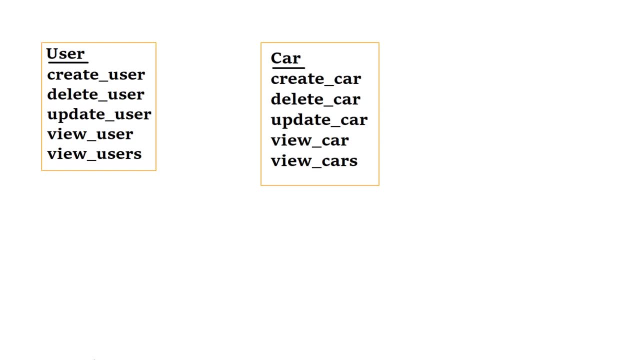 you can set a routine for you, Save of information or create a location from the location. We will import this data to our REST API and we are going to send you on a list. Yes, the resource will be having different roles. he can be a normal user who wants. 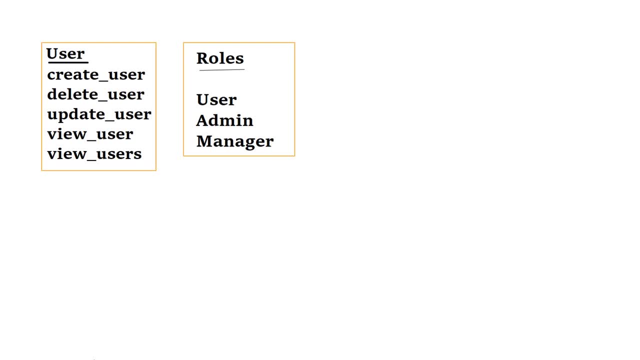 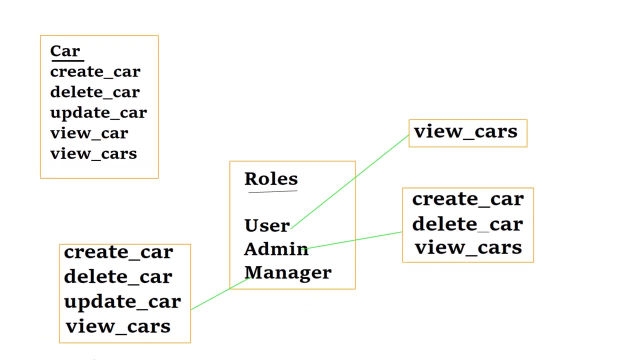 to see all the cars available. next, the admin- one who is responsible for creating or deleting the resource, and also the manager. depending on their roles, they will be having different set of permissions. for example, for the car resource, the user will have only permissions to view the cars he can view. 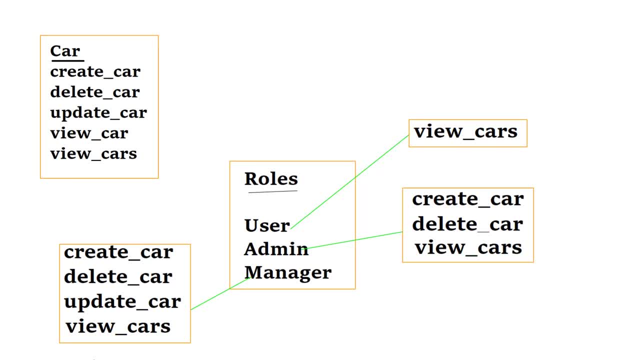 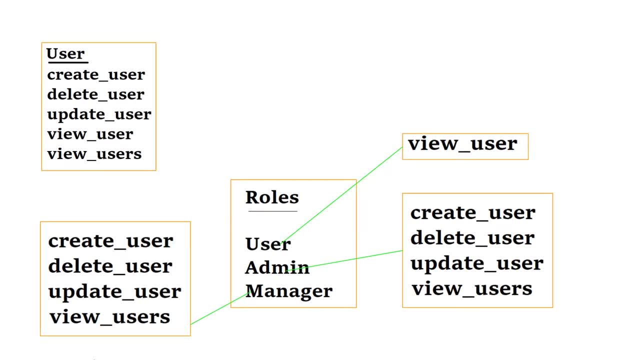 the cars, but the admin or the manager will have permissions to create, delete and also to update the car resource. similarly for an user also, the user can view only his own details. he cannot view the details of any other users. the admin and manager will be having all the other permissions to. 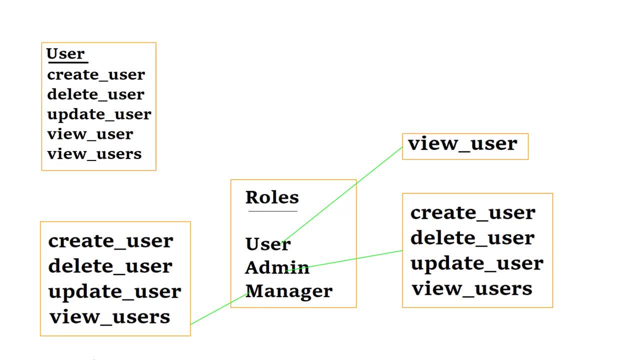 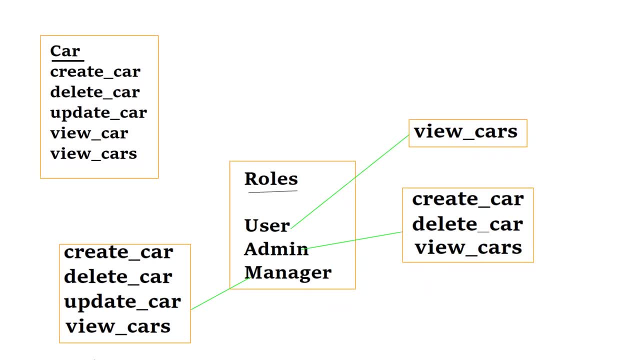 create, update, delete and view other users too. this user object is used for authenticating the users who comes down productions in for the car resource, We are going to implement the same. We are going to control the access to the resources based on the user's role. Let's see how to implement this using this spring security. 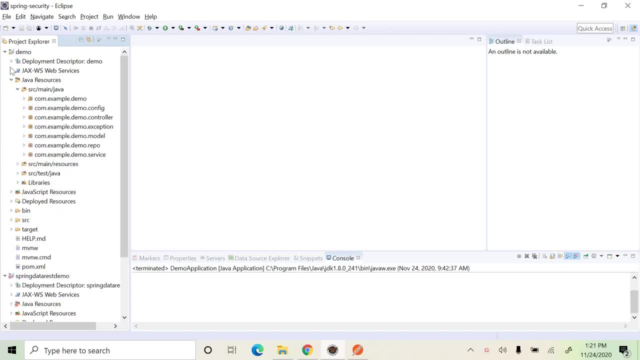 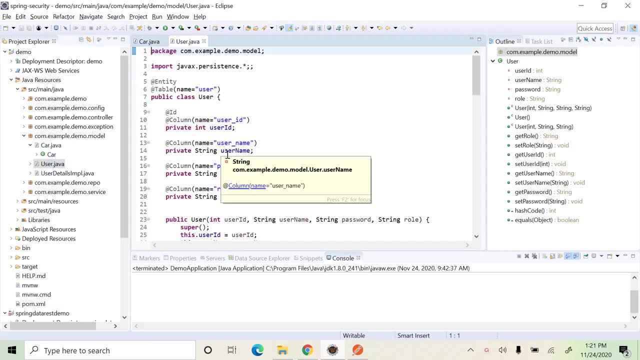 I have imported the sample application into Eclipse. First we can see the domain objects. There are two domain objects: car and user. This car is the resource which we are going to access and this user object is used for authentication purpose. So the user has user id, user name. 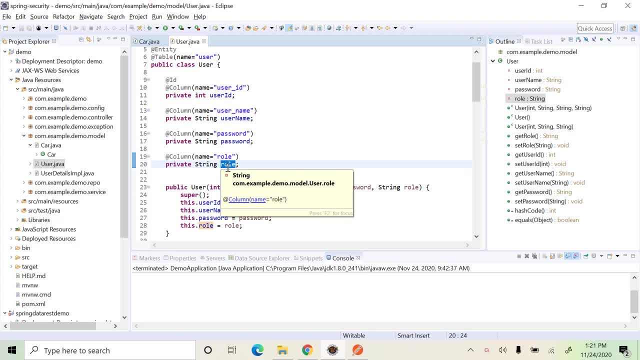 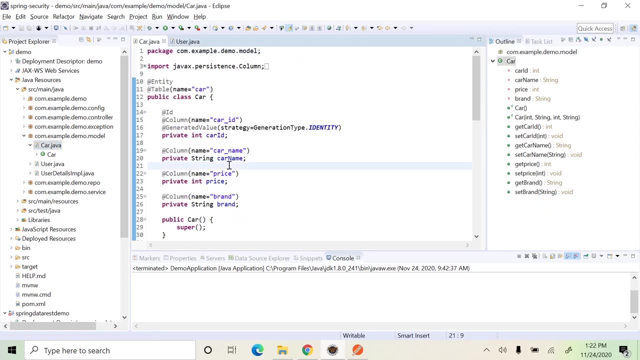 password and a role. Each user is going to have one role: admin, user manager, editor, like that. Each user is going to have only one role. and here is our car object, which takes an id name, price and brand. We have to create the repository. 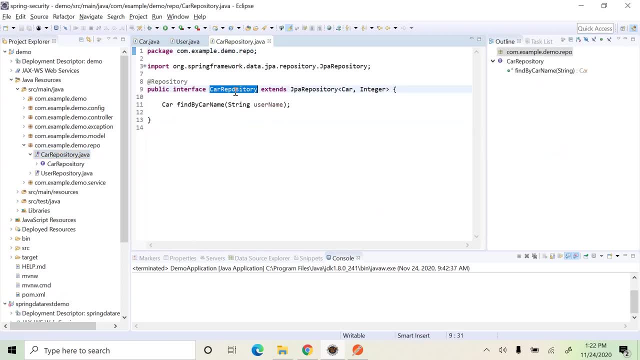 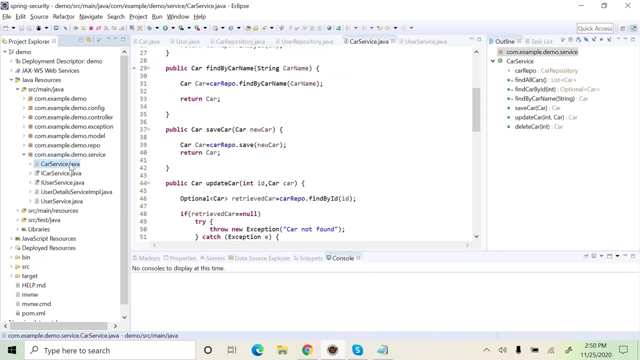 Now there are two commenting birthdays for this. two domain objects: car repository, which is a JPA repository to access the database, and an user repository for the user object. Next we have to create the services. We have two services: a car service and an user service. 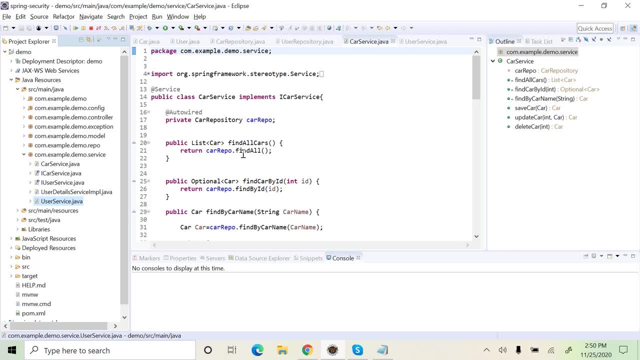 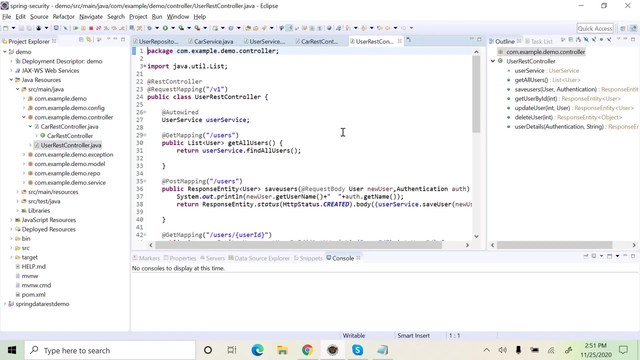 which contains all the methods to do the save, update and retrieve operations of this car object and user object controllers too. we have to create the controllers for this car object and a user object. these are rest controllers, which serves the incoming request to the rest endpoints. we are done with the rest. 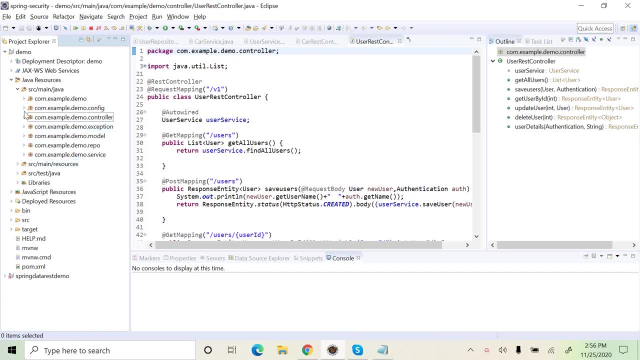 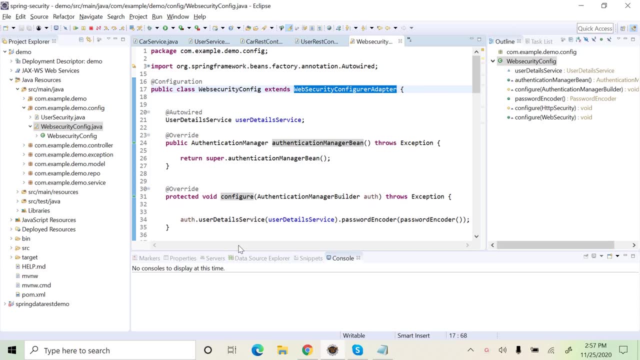 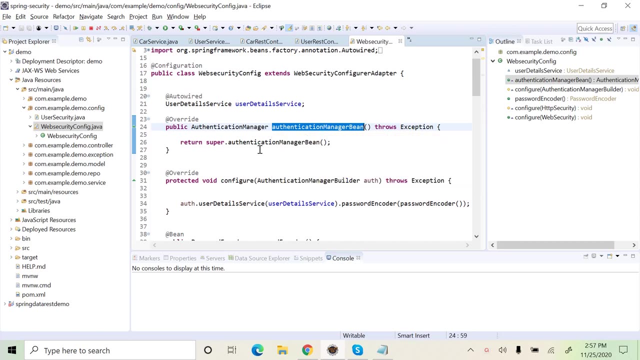 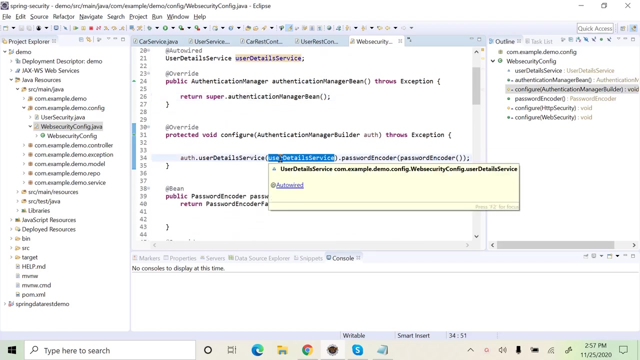 API stuff. next, we have to configure the web security for this rest API. so we can do that by extending the web security Configurer adapter. here we have to overwrite three methods: the authentication manager bean- we have to return the authentication manager bean from the super class- and then we have to give the user details- configuration for authentication, along with 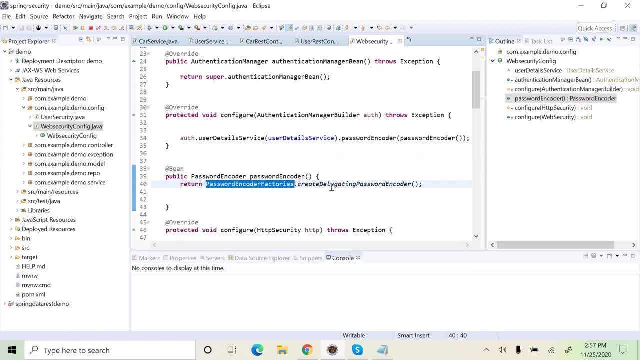 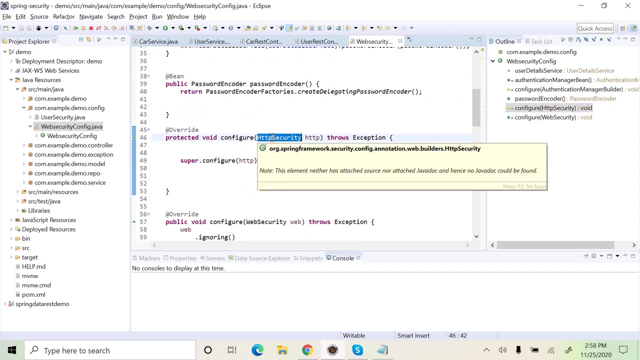 the password encoder. here we are using the create delegating password encoder, which returns the password encoder from the password encoder factories. and this, this configuration, this authentication manager builder configuration, is for authentication purposes. next, this authorization related configuration is done in the HTTP security. let's run the application without any authorization configuration and see how it works, and later we 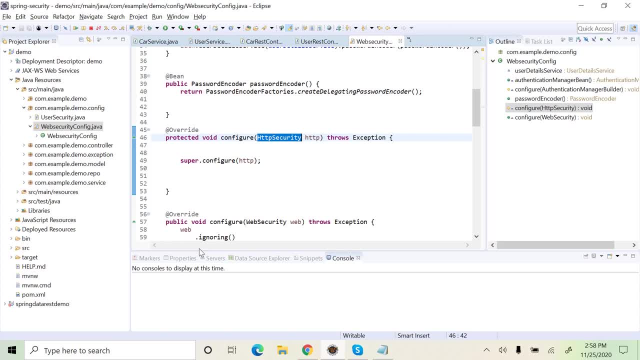 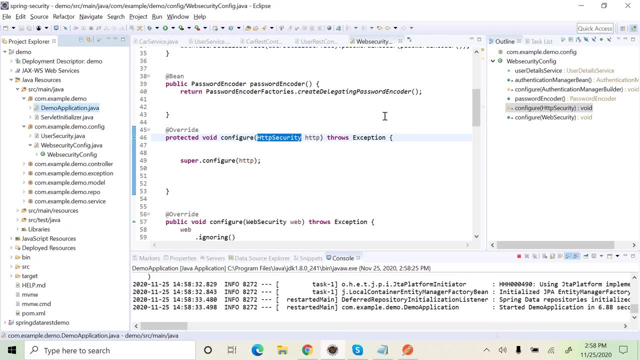 can add the authorization related configurations and see what makes a difference. let's run the application. we have configured web security here, so each and every request must be accompanied by the authentication related information, that is, either the username or password or tokens- whatever is necessary to authenticate the user. the application is running at port 8080 and this is the endpoint. 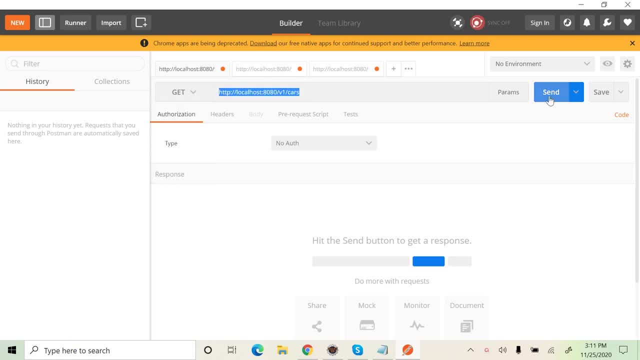 to retrieve all the cars, get method is selected, let's send this request. we are not giving any authentication information here. that is username or password. it doesn't carry any authentication information. now we are just sending that request. so it says 401 and authorized, because the request didn't have. 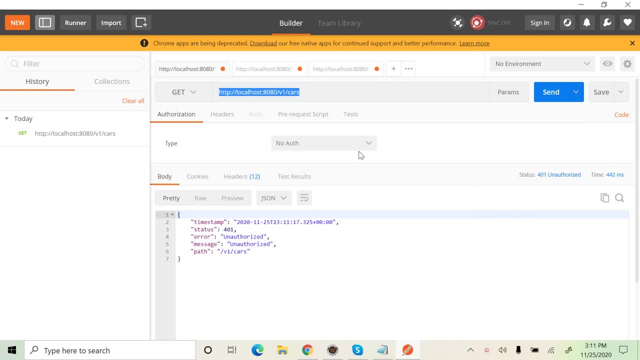 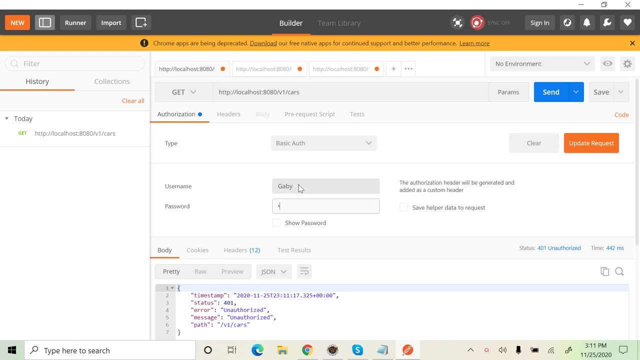 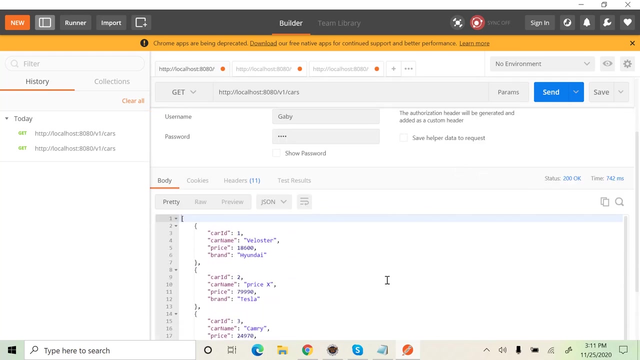 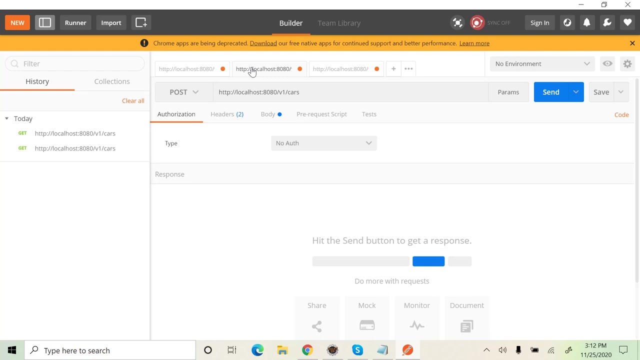 any authentication related information. now we can just select the basic authentication and give the username and password. let's resend the request. we have retrieved the cars from the database which say gives a 200 okay, and it returns as a list of cars from the database. now we can try the post method to save an car object into the database. 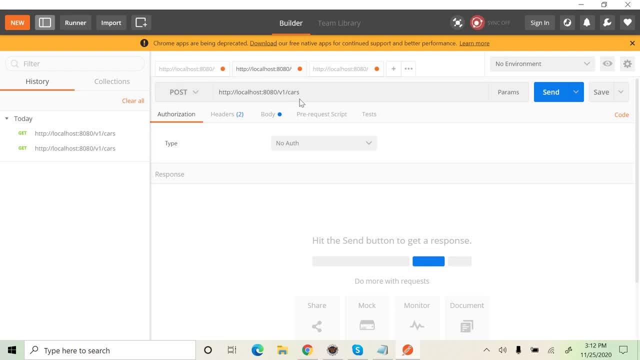 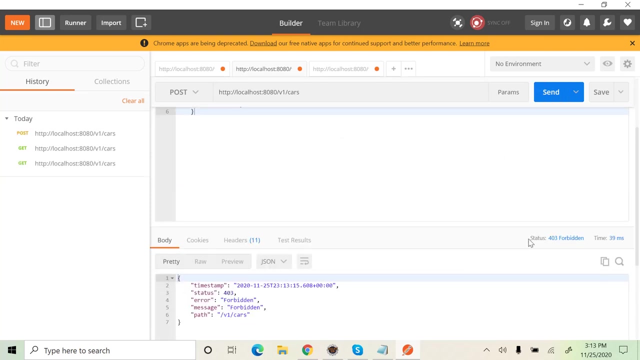 we have selected the post and this is the endpoint to save a car object and in the authorization we have to select the basic authentication and give the username and password. and in the body section you have given a our object in Json Format. let's send this request. it says 403, forbidden. we have given the authentication information. 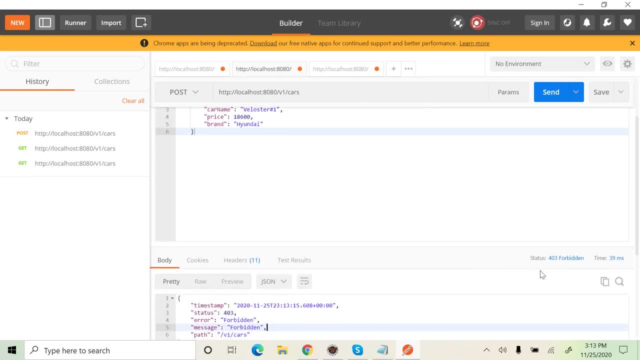 like username and password. in spite of that, we get a 403 forbidden. this is because by default spring security You wrist cap or you aren't. anному xxpo for Archivesamps is something else has enabled the CORS restriction, that is, cross origin resource sharing restriction and cross. 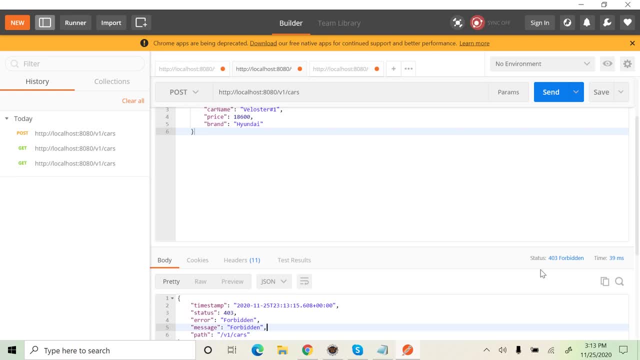 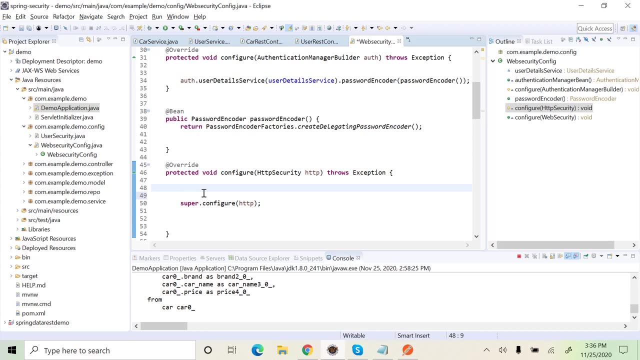 site forgery restriction in order to prevent the attacks from a different origin and a different site. To remove these restrictions, we have to configure the CORS and cross site forgery restrictions separately, just specifying where, from which origin and from which sites resource sharing can be allowed. But for here, just for learning purposes, we are going to disable it. 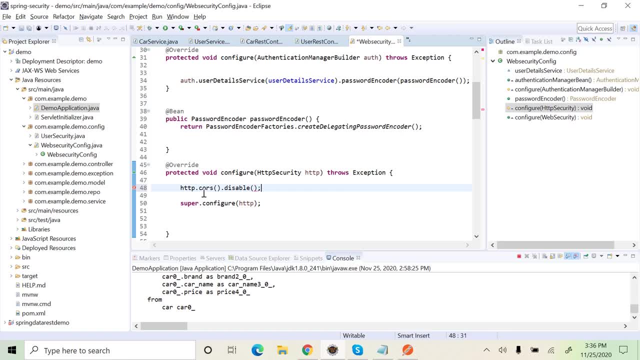 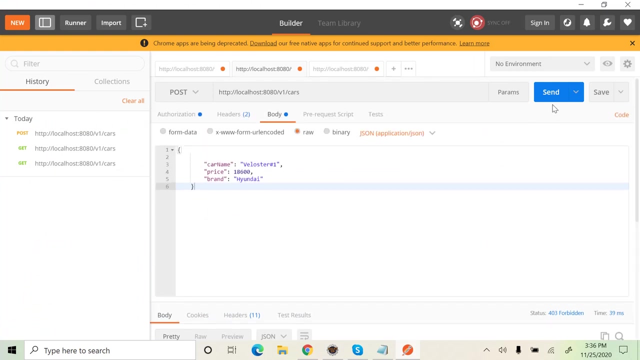 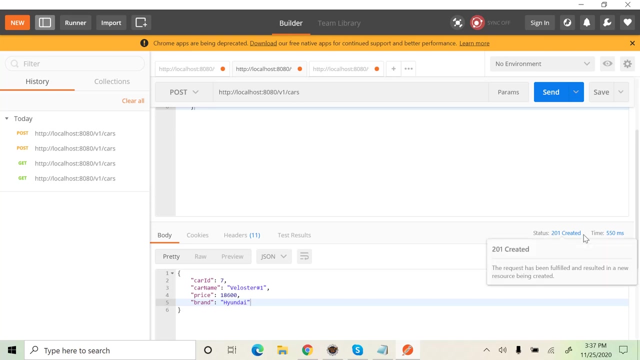 http course disable: this will disable the CORS and http csrf disable: this will disable the cross site forgery restriction. Now let's resend the request. same request After disabling both CORS and csrf. we are just resending the request. Now it gives a 201 created. 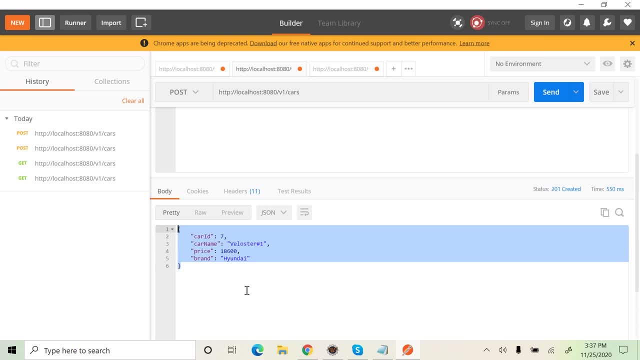 response along with the saved COR object. Likewise, the other operations, like put, delete, also works along with the authentication information. Here we haven't given any access control, that is, we didn't authorize any user. here All users can access all the endpoints. All users can access all the resources. They have the permission to do all the. 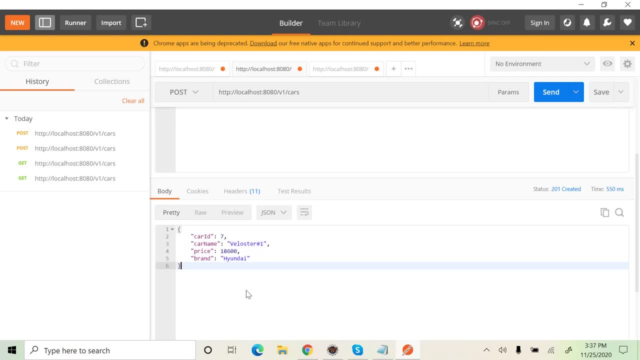 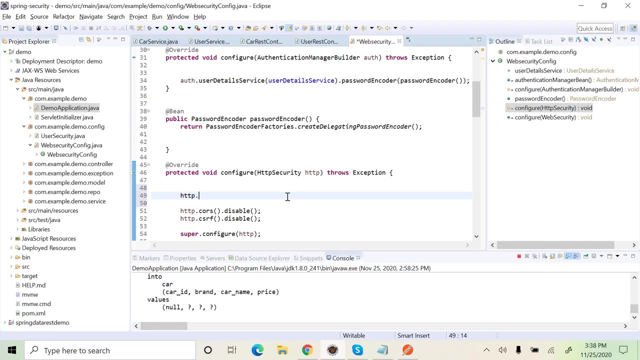 operations on the resources. but this is not how it works. Each roles should have a specific permission to do specific operations. Let's go back and configure this in http security httpauthorize request. All the request has to be authorized Initially. it will be authorized as GCSE BUT 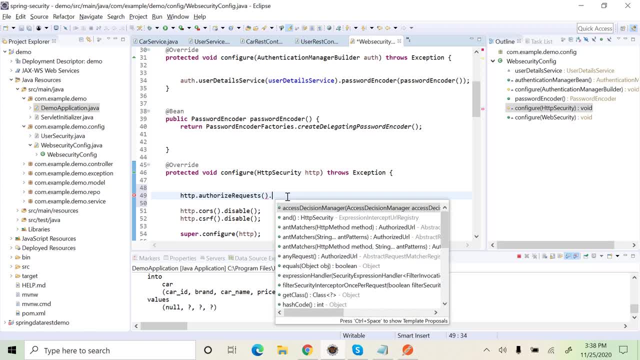 we don't need a request response, so we just complete it and make it as a about: Nah, The renewal is 로 tolt rf, so it is going to include another solution which we are going tolik rfnot off without Remove from SOAP. I type what we. in You can check the RM Rams and any other data you want to run. You would want them from some good runningplease, Whereas in My BIOS you can put some command serie wishよね. So let me just echo this,343 and then click enter declared Wita. 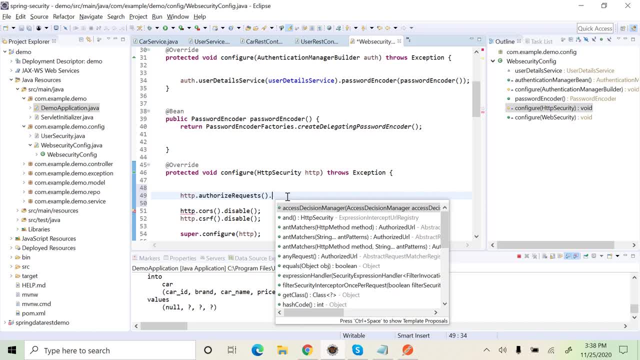 be authenticated. here we say that it has to be authorized to, and we are going to authorize based on the http methods. we are just going to see which roles are going to have access to which http methods. let's start with the post method and the matches, and here we have to pass in the 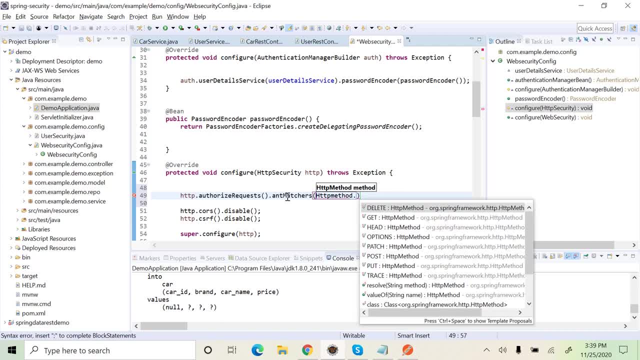 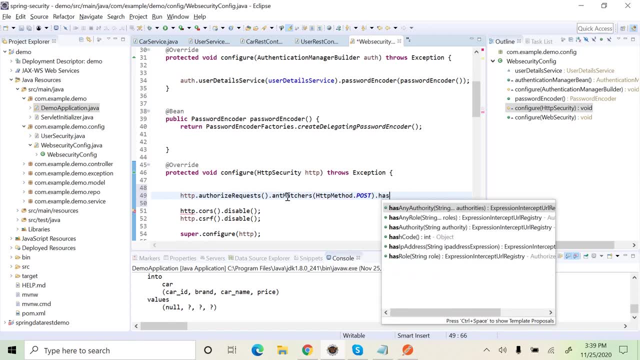 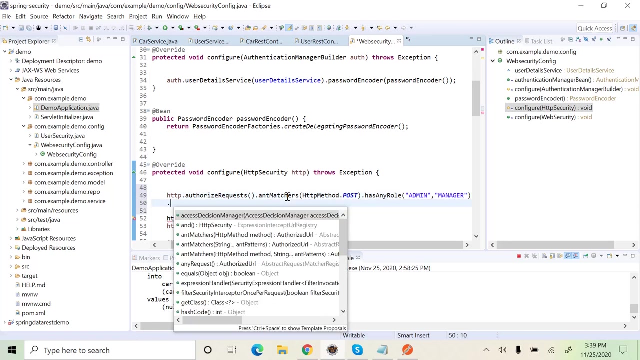 http method post method. this http post method can be accessed by any roles, like admin and manager. similarly, we have to configure for all the the http methods too. here post method will be accessible for all the other https methods. also, here post method will be accessed for all the. 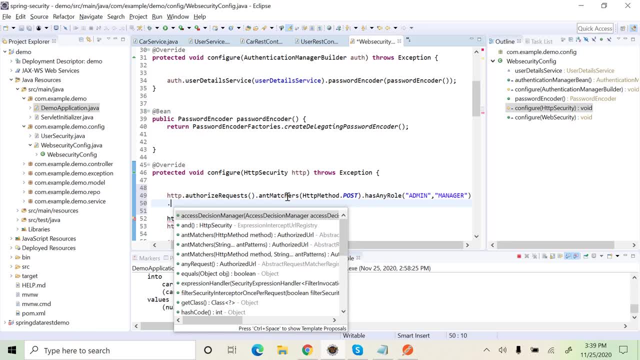 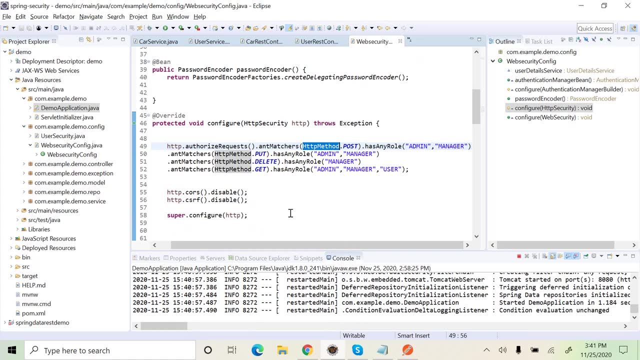 blushers. also here, post method will be accessed for all the others, etc. so let's start with the post method by the users who are having the role either as admin or manager. here we have configured the access control for all the HTTP methods: the post and put method. 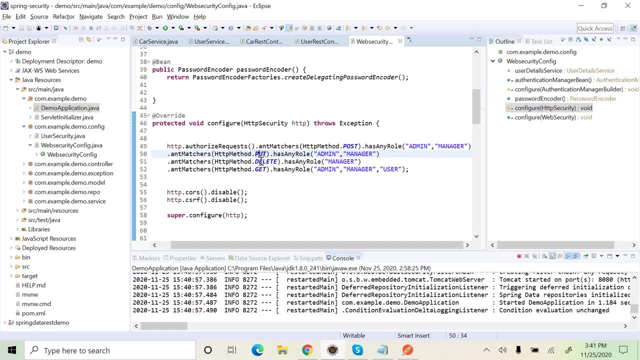 can be accessed by admin and manager. the delete method, that is, the delete operation, can be done only by the manager and get can be done by all the users: admin, manager and user. let's now go back and check whether this authorization stuffs work or here. initially, the post operation is done by: 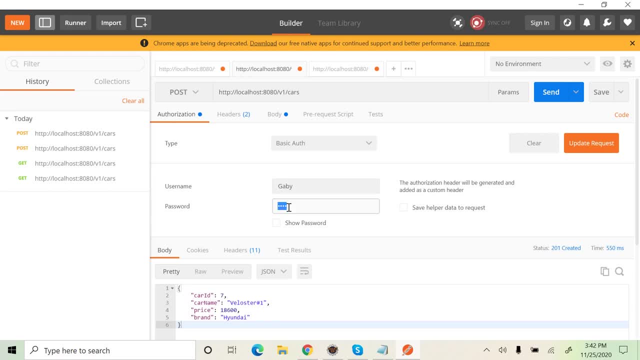 a user who has an user role, but according to our authorization information, a user role cannot do the post operation. now let's check whether this user with the user role is able to access the post method after the authorization has been completed. the configuration: no, this user with the user role is not able to access the post. 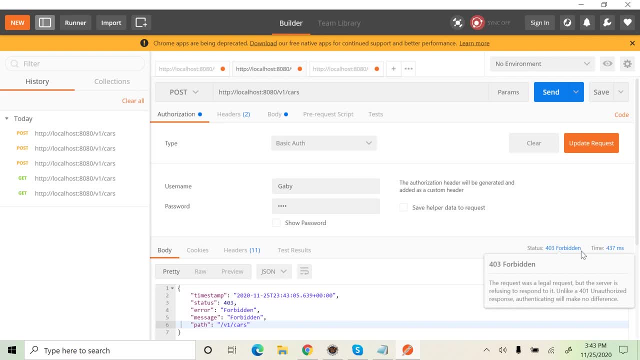 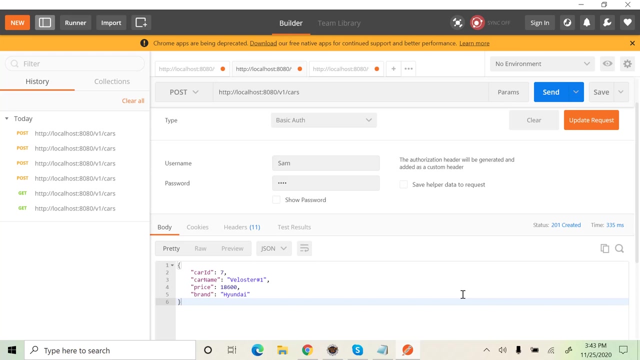 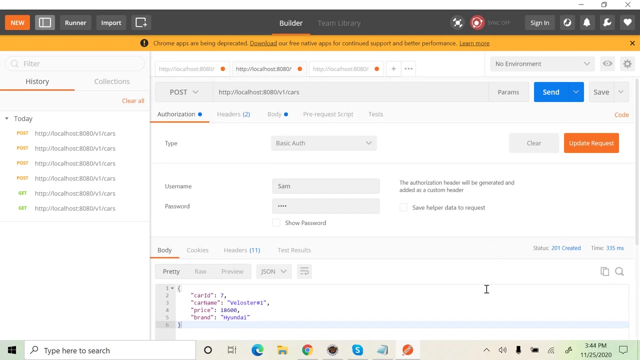 method, it gives 403: forbidden because this user doesn't have the permission to access the post method. he doesn't have access to update the database. let's try with another user who has a admin role. yeah, the user with an admin role is able to save a resource, that is, the user is able to access the post method. so this: 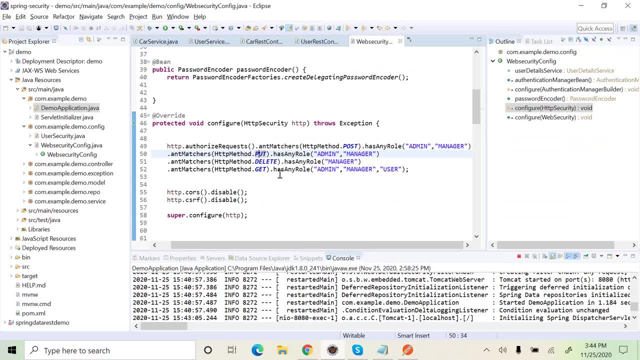 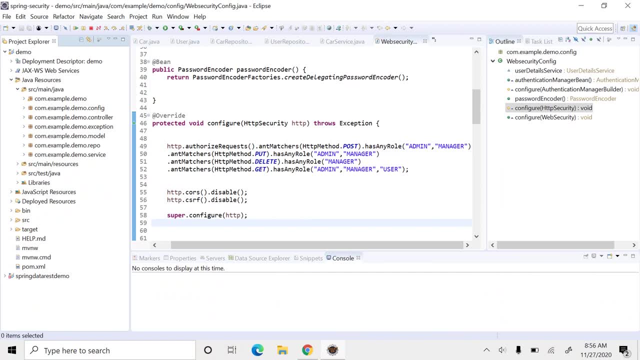 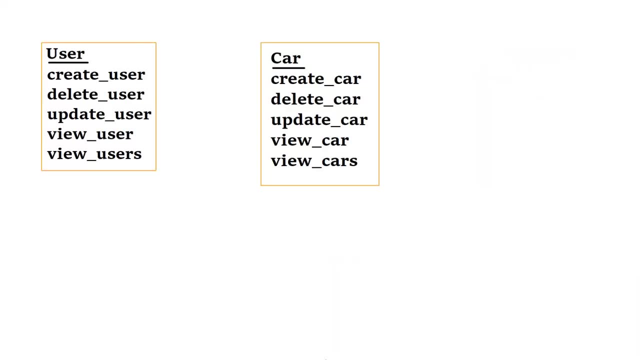 is how authorization works. here we have configured the access control based on the HTTP methods. in this application, we have applied the access control by HTTP methods. we have applied the access control by on the HTTP methods. But according to our application, we have two resources: a user. 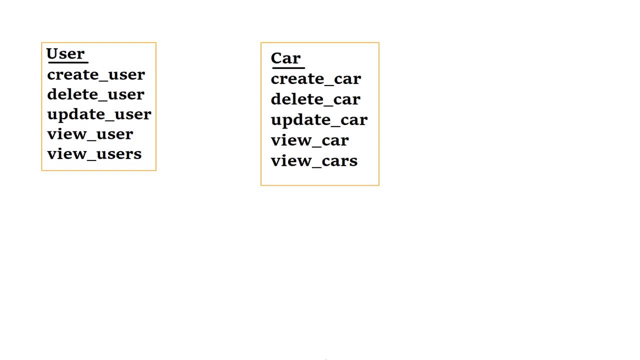 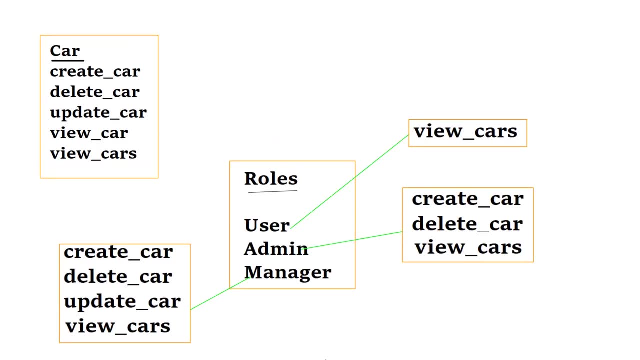 resource and a car resource. Both cannot be accessed in the same way, because a car resource will be accessed in a different way when compared to a user resource. If you take the car resource, the user can view all the cars, But whereas if you take the user resource, the user can view. 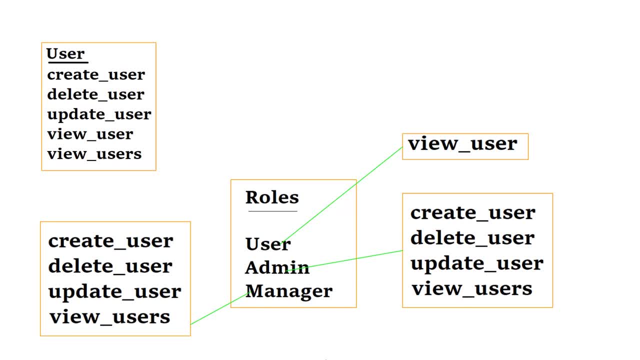 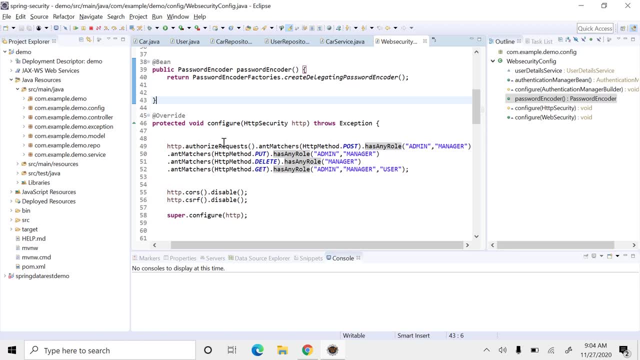 only his own details. He cannot view all the user's details, But according to our configuration, both the resources will be treated in the same way. That is, we have applied the access control based on the method level, So both the user resource and the car resource will be accessed. 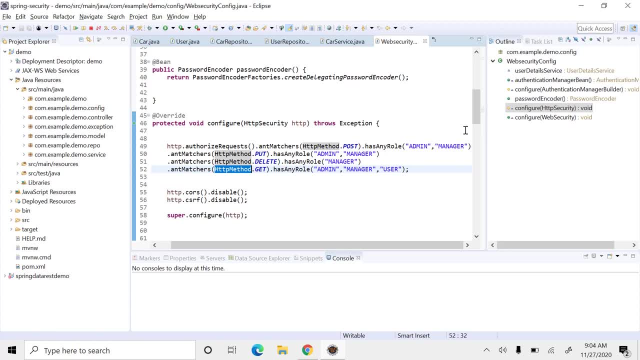 in the same way. So we have to fine tune it. For this, what we have to do is we have to apply the restriction at the endpoint Level 2.. We have to fine tune it from the method level restriction to the endpoint level. 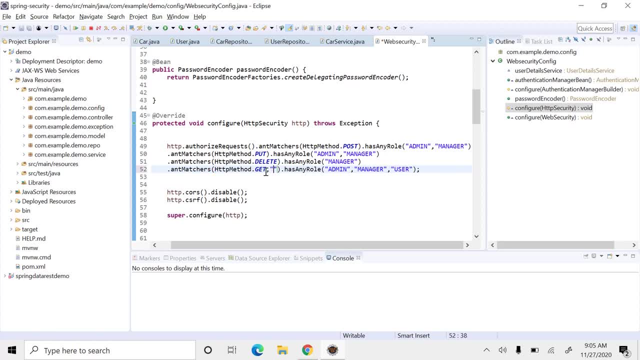 restriction. For this we have to give one more argument, which is the endpoint. slash v1, slash cars is the endpoint to retrieve all the cars, And here we have to specify: it can have any role, like admin, manager and user, Whereas the user's endpoint, which 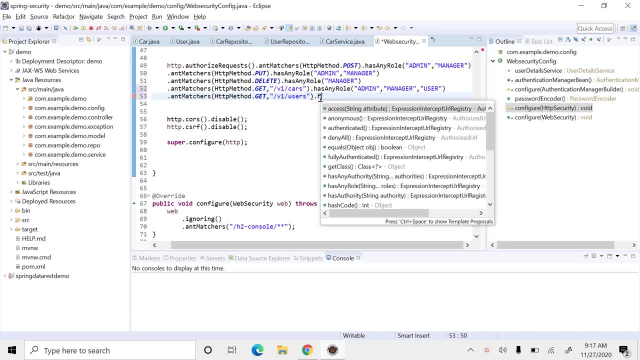 retains all the cars. So we have to specify it can have all the cars. And here we have to specify it can have all the users. details must be accessed only by roles like admin and manage. Now we have just fine-tuned it to the endpoint level. Now the cars endpoint, which returns all the cars, will be. 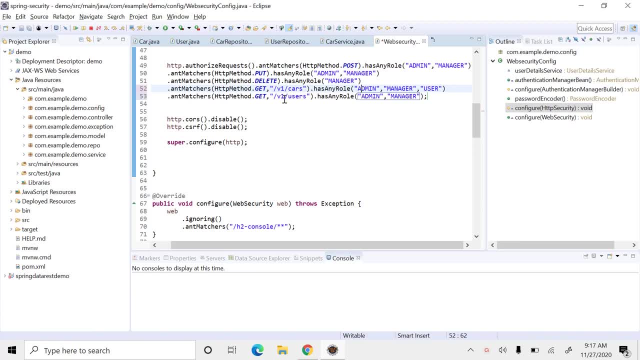 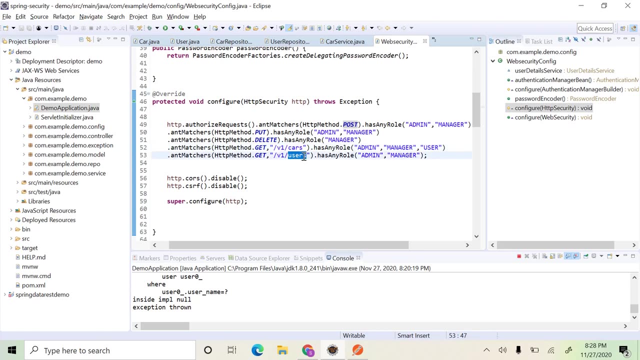 accessed by all the roles, whereas the users endpoint, which returns the details of the users, will be accessed only by the admin and manager. Let's test these two endpoints- cars and users- to see whether it is authorized properly. So this is a cars endpoint to retrieve all the cars. 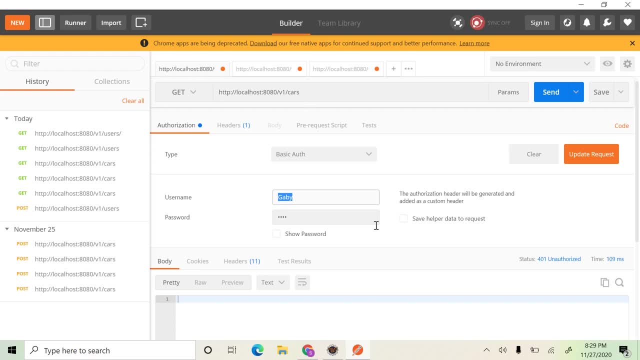 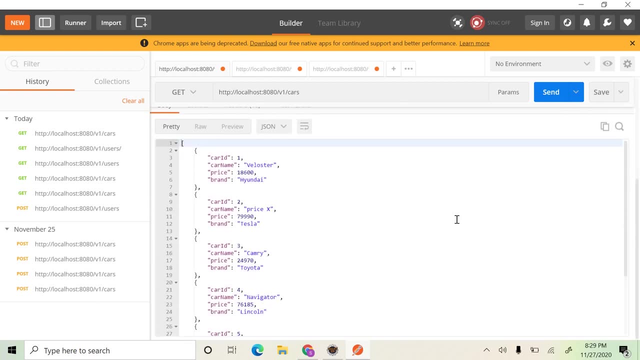 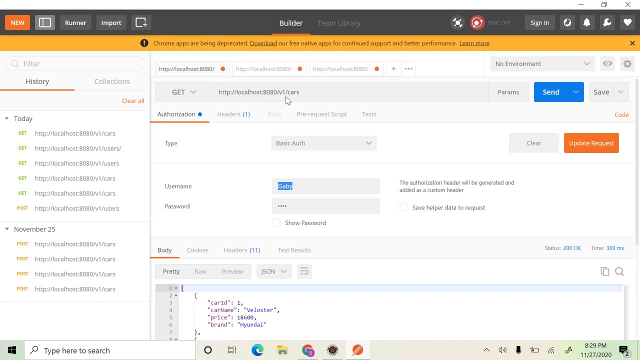 and Gabby is an user who is having the user role. Let's send the request and see what happens. So now we are able to see all the cars. It is retrieving all the cars. An user with an user role is able to see all the cars. Let's call the users endpoint to see a user with an user role is. 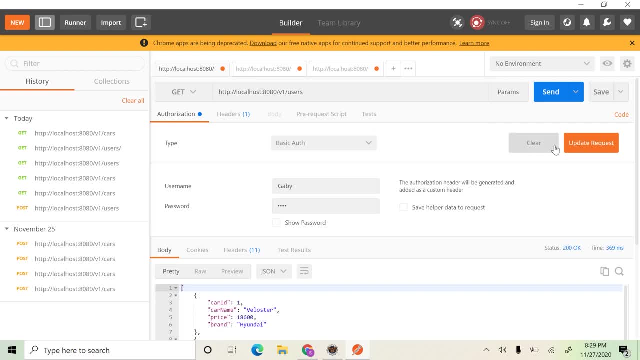 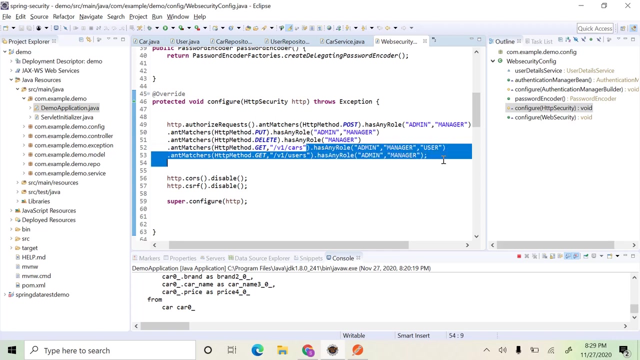 able to view the information of all the users. No, it gives a 403: forbidden because the because the user who has an user role does not have access to this users endpoint, which retrieves all the users details According to our authorization configuration. But the user should be able to view his own details. 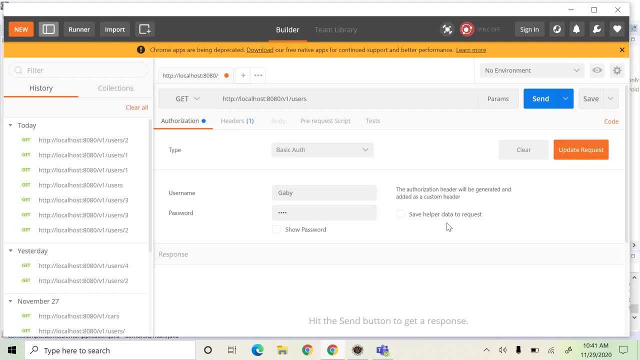 That is, whenever the user passes his own ID, he should be able to view his own details. So let's check whether it works. The users- Gabby- has a user ID of 2. Let's send this user ID and see whether Gabby is able to get the details. 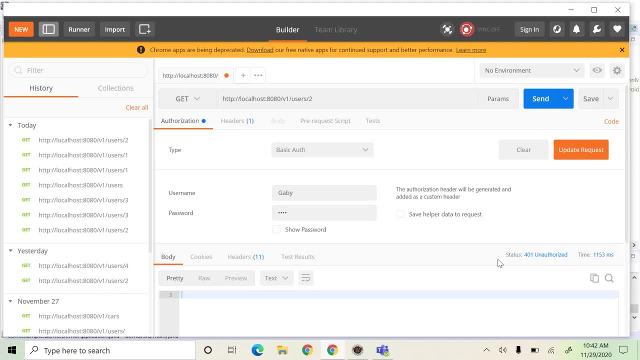 No, Gabby is not able to retrieve the details because we didn't configure that endpoint. We have to configure that endpoint such that the user should be able to view only his own details. To ensure this, the incoming user ID should be validated against the authentication information. 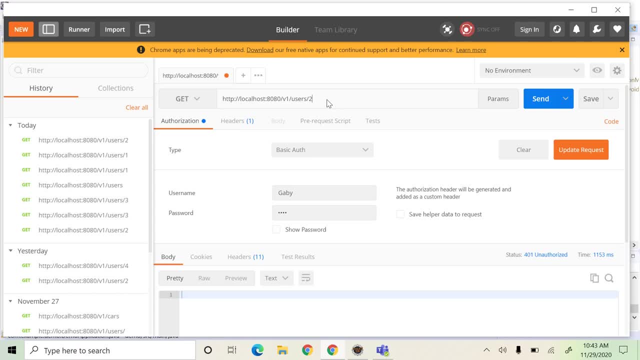 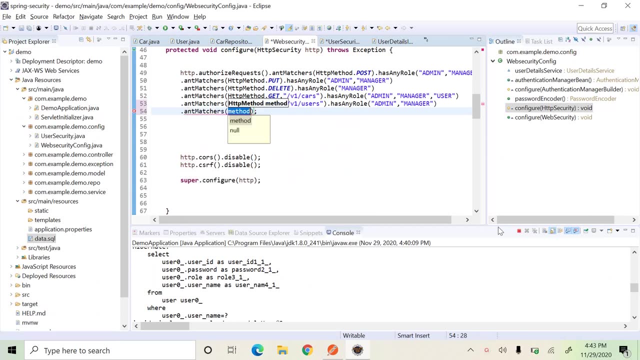 that is, user ID that comes in must be equal to the user ID of the currently authenticated user. Configure this endpoint to see the user ID of the currently authenticated user. We should again use ant matches: gtpmethodget. user endpoint v1: slash users: slash user ID. 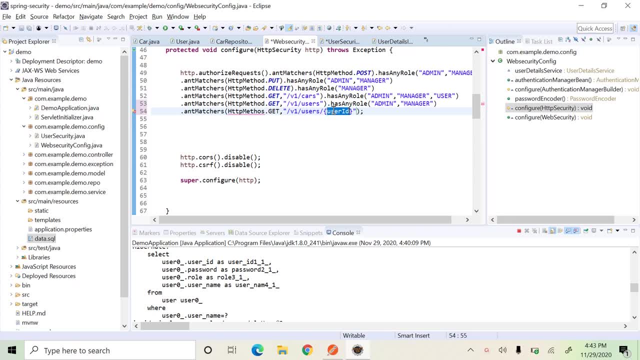 This user ID is a path variable. Here we pass in the user ID of that user and this user ID has to be verified against the user ID of the currently logged in user. The currently logged in users information will be. that is authentication information will be stored. 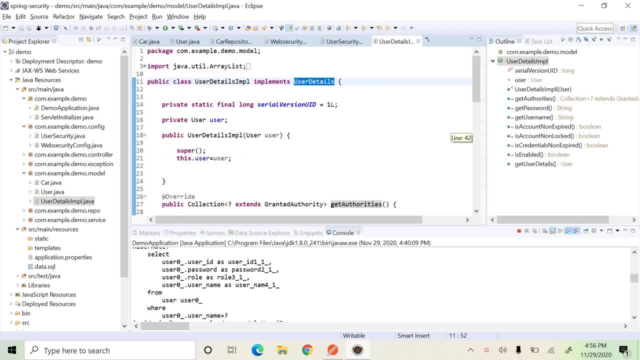 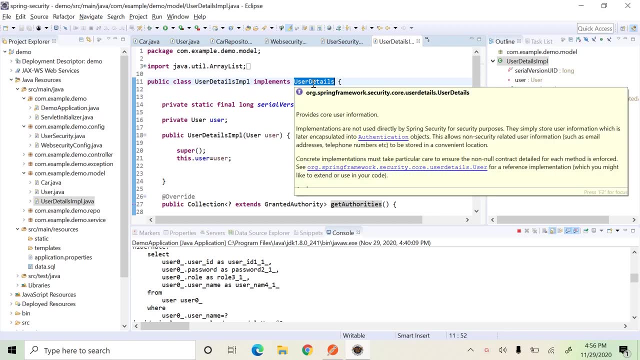 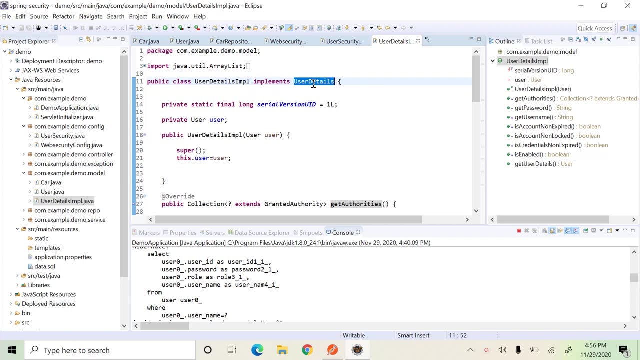 in the security context holder and this authentication object is created by spring security when it authenticates an incoming user and this authentication object contains this user details object within that, that is, these user details object, is encapsulated within this user details object The authentication object. so using that authentication object we can get the user details, like username. 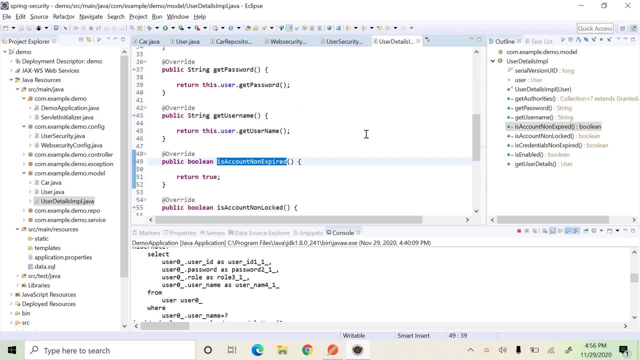 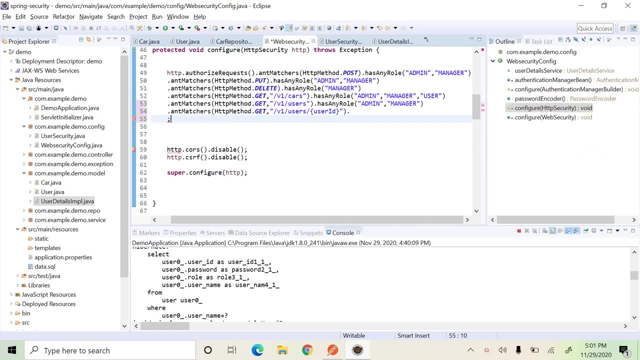 password and the roles of that user and other data that are required to authenticate an user. We are going to make use of this authentication object to validate the incoming user ID against the user ID of the logged in user, that is, the user who is currently authenticated for. 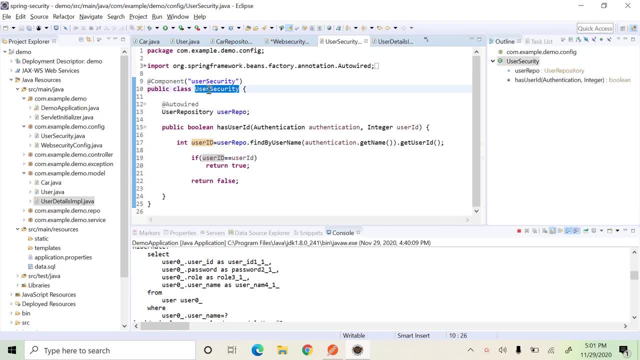 that we need to create a new component: user security. in this class we have a method called has user ID. this method takes an authentication object and the incoming user ID and it validates whether the user ID is equal to the user ID of the currently authenticated user. it does this by: 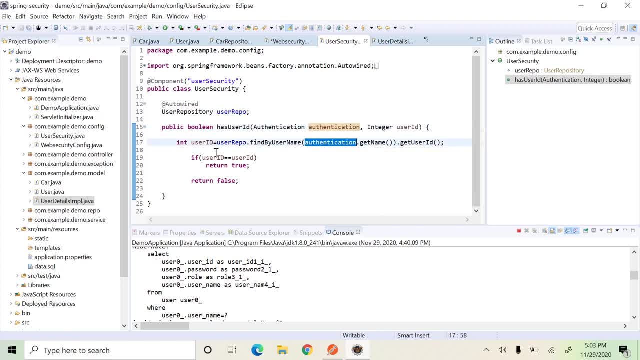 retrieving the user name from the authentication object and retrieves the user ID of that particular user And it validates against the user ID that came in the path variable. if both the user IDs match, it returns true, otherwise false. so when it is true, when this method returns true, 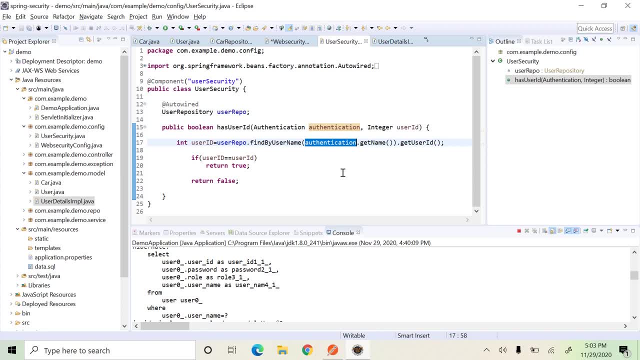 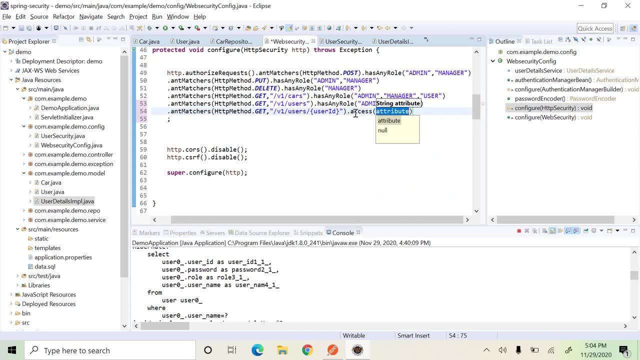 the user will be getting his details, otherwise it will return an error response. we have to configure this here: dot access and it takes in the expression at user security. that is the component and you have to specify the method name here has user ID and we have to pass in the authentication. 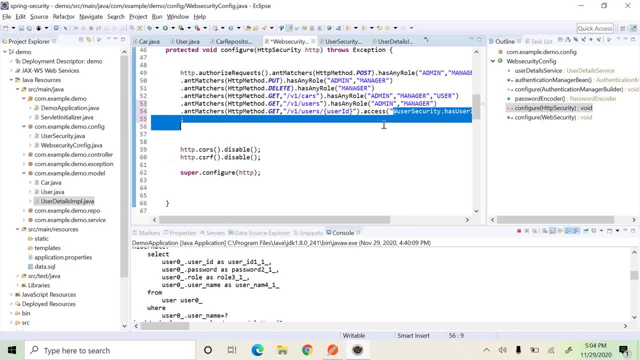 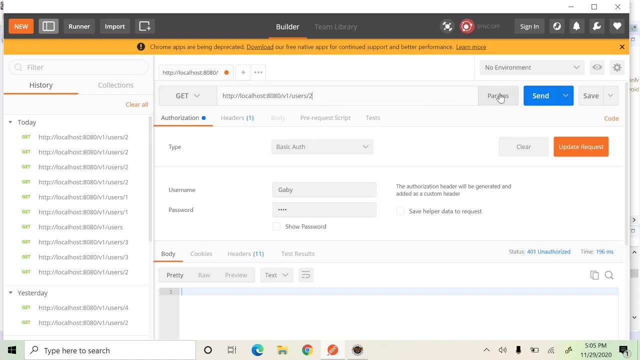 and user ID. we just say that if this expression is true, the user will be given access to this endpoint. otherwise, he will get an error message. now let us test whether it works. Gabby is an user with the user ID 2. let's send the request and see whether we are able to view the details. yes,